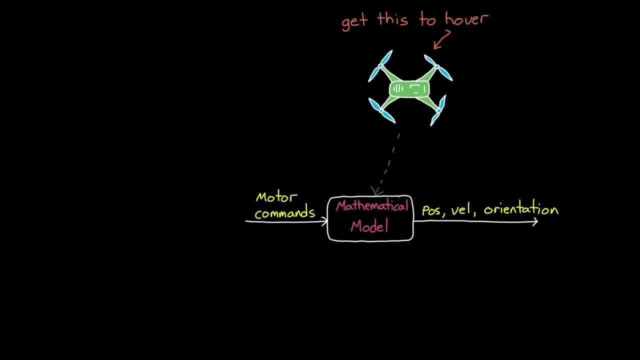 to outputs, which is drone position, velocity and orientation. You know, basically some function that mimics the behavior of the real drone, And then you use that model to design a controller, which is just another mapping that takes a reference signal and a system state as inputs. 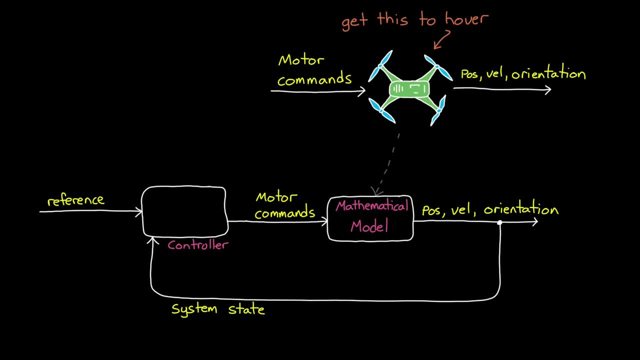 and then outputs the controlled variables. And these are the things that we can use to affect the behavior of the process. And this controller mapping can take many different forms. It could be PID or full state feedback, or a neural network, or some nonlinear mapping, or whatever you choose to solve your problem, And you probably have some. 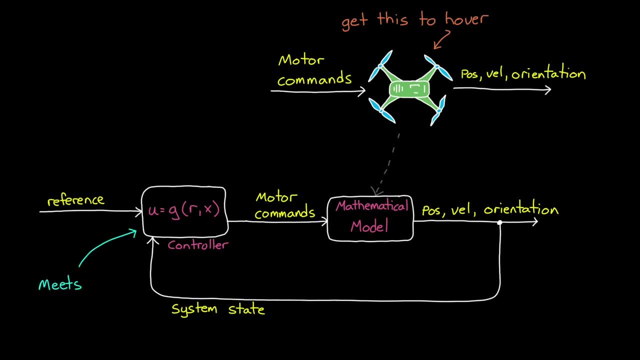 performance or stability requirements that you're designing to, And once you have a controller that works with the model, you can implement it on an embedded processor that drives the actual drone, And if your model was close enough to the real system, then you have some expectation that the 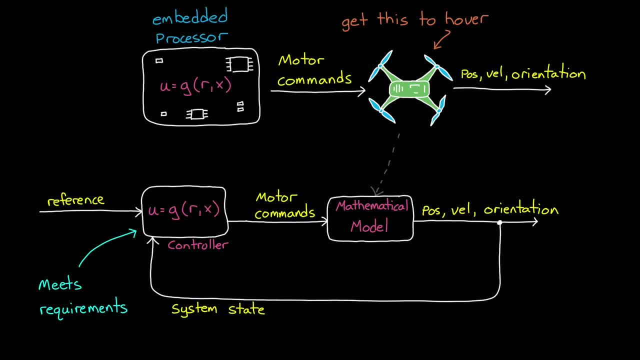 controller you designed will work on the actual drone And if your model was close enough to the real system as well. But here's the sad reality: Your model, the model you use to design your control system, is wrong, which means the control system isn't going to work. exactly the same on. 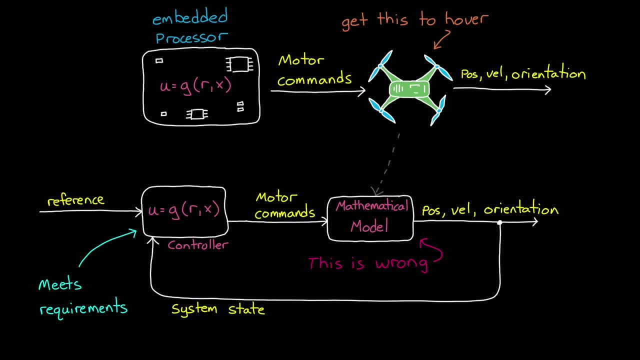 the real hardware, as it did against your model. Now the main question is: is it good enough, though? I mean, our controller could probably handle some differences in the real system right Well, before we address that, let's look at why the model is wrong in the first place. 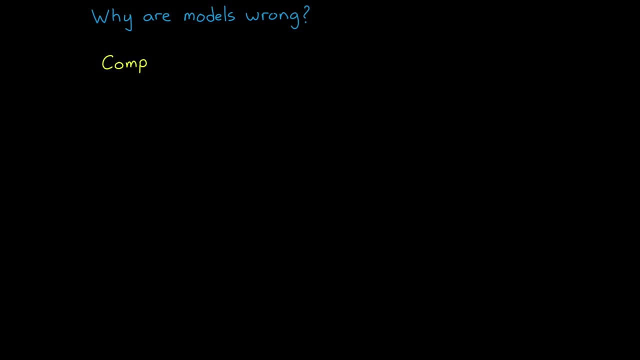 And there's lots of reasons. Real systems are extremely complex and the input to output mapping may be poorly understood. For example, we may not understand or be able to measure certain things like high frequency dynamics. Therefore, our model won't include them, or at the very least, 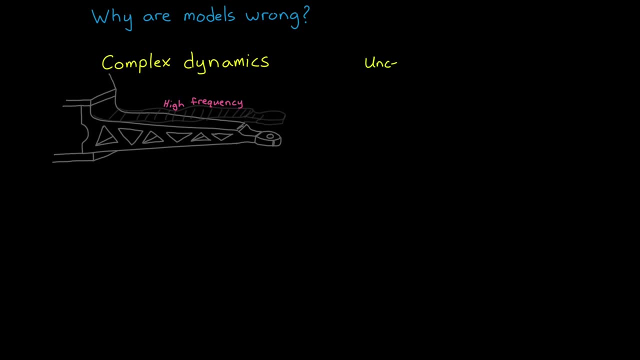 they won't be accurate at these frequencies, Or we may not understand the inputs into the system very well, Things like disturbances or even the behavior of our own actuators that are driving the system. So there's a lot of reasons why the model is wrong, But if you're a real system, 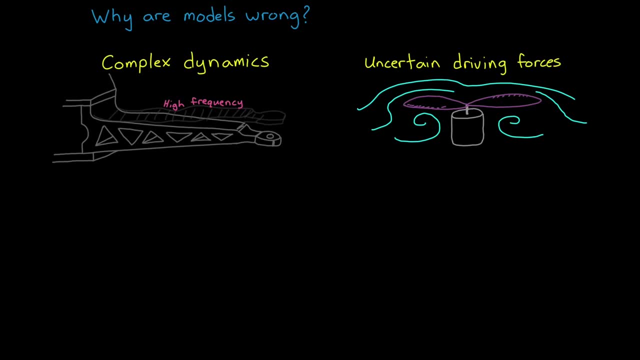 there's uncertainty in both what the driving forces are that go into the system, as well as uncertainty in how the system responds to those driving forces. Now, additionally, we may also intentionally build a model that deviates from the real physics in order to get something simple. 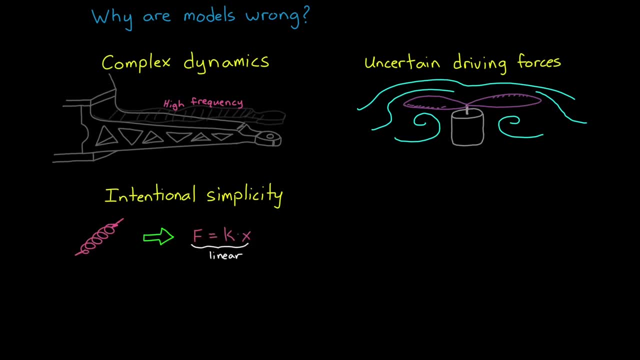 to work with. This is the case for every linear model. We've sacrificed realism for simplicity. Another thing is that the system itself may naturally vary over time and the changes driven by unknowable stochastic events. Short-term unknowable events we might label noise, whereas 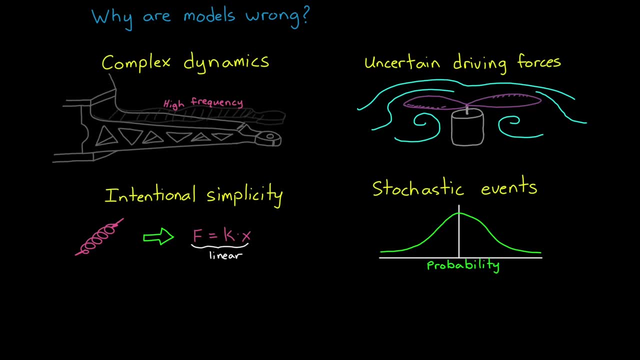 longer-term events might be things like how the system degrades over time. The drone might not behave the same brand new as it does a year later. And finally, you may be designing a single physical system, but manufacturing tolerances and defects means that you don't exactly know the parameters. 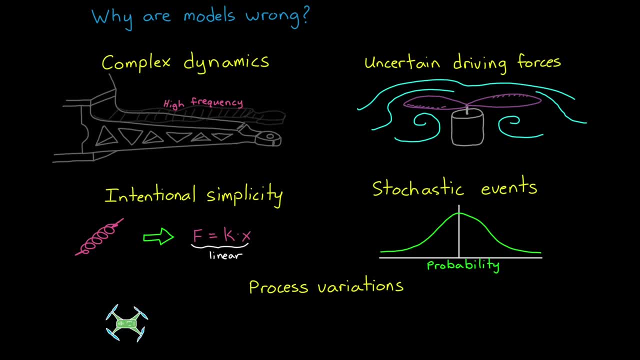 of duplicate systems. Say, for example, the controller is for a toy drone that you're selling, but each drone is manufactured slightly differently and so each flies slightly differently. A single system model wouldn't capture the uniqueness of each of the drone variations and therefore would have some amount of error when we use it to represent the set. 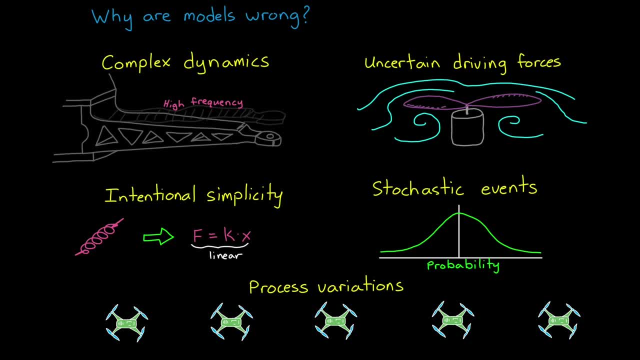 of all of the drones. All of these things make models, imperfect representations of real life. They're just approximations, but they're extremely helpful to solve many problems. so we're willing to put up with the fact that they aren't perfect, But because of their imperfections, 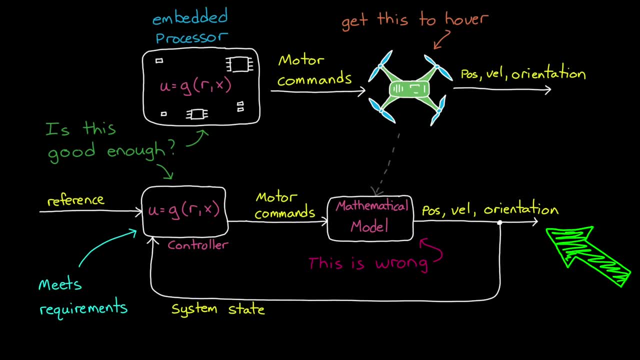 there is some uncertainty, some unknown difference between the output of the model and the output of the real system. Therefore, when you use a model to design a controller, the consequence is that it's being tailored to an imperfect representation, And so a controller that is perfectly tuned to the 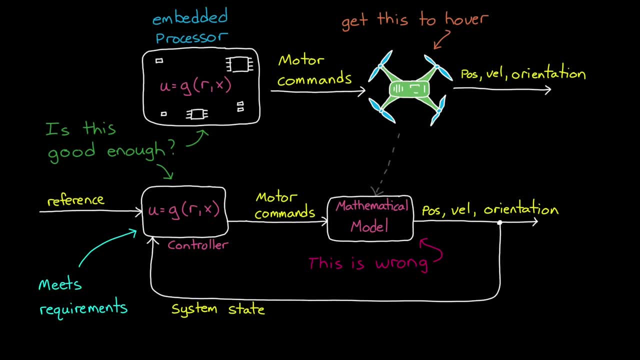 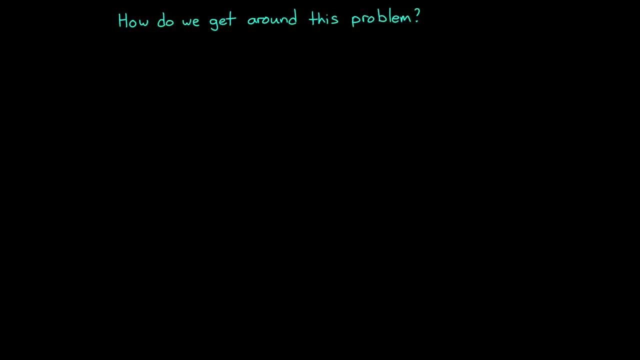 model still runs the risk of reduced performance or reduced stability on the real system. So how do we get around this problem? Well, a straightforward way is to simply add margin margin, For example. don't just meet stability, but exceed it by a certain amount. some margin. 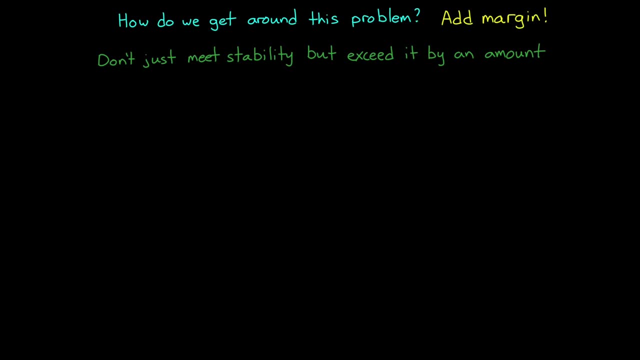 so that we're confident that any deviations from what we think the system behavior will be won't result in the system exceeding a requirement. We're just going to eat into some of that margin. If you're familiar with the classical gain and phase margins, this is exactly what they are for. 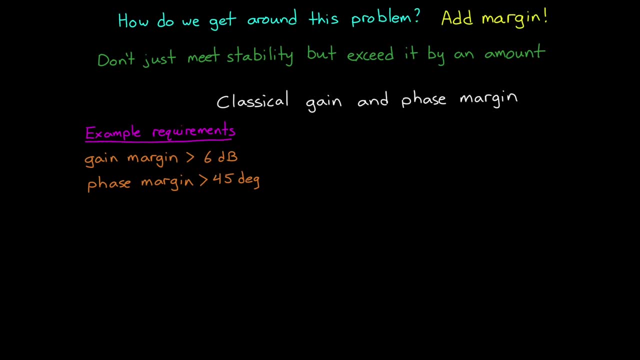 You may have a requirement that says gain margin must be more than six decibels and phase margin must be greater than 45 degrees at some critical frequency. If you're familiar with the classical gain and phase margins, this is exactly what they are for. You may have a requirement that says gain margin must be more than six decibels. 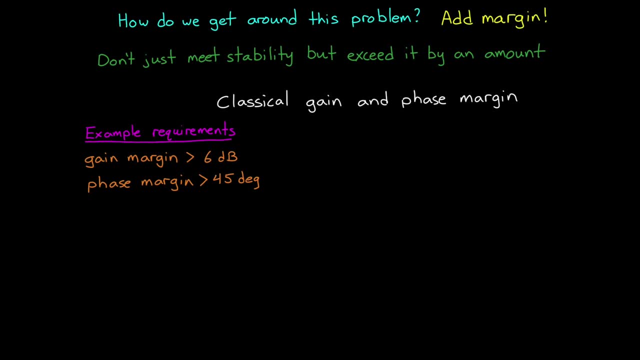 and phase margin must be greater than 45 degrees at some critical frequency or frequencies, And what this is saying is that you have to design your controller in a way that the real system will still be stable, even if the gain is up to six dB higher than your model claims or if the phase 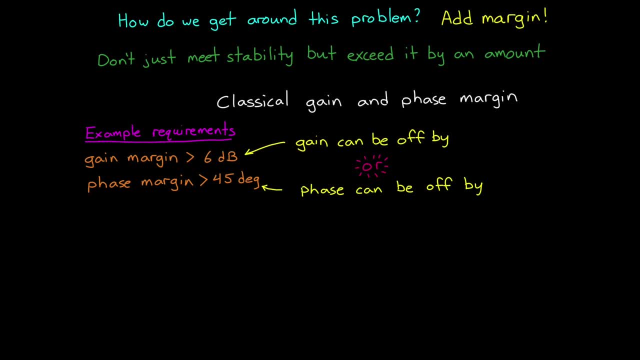 lags up to 45 degrees more than your model claims at the frequencies that it's specified at, And choosing the amount of margin you need depends on how uncertain you are that your model matches the real system. If we choose too little margin, then the differences between the model and the real 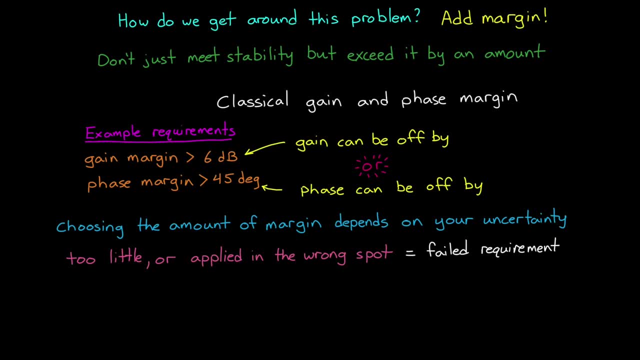 system may cause a lot of problems. So if you're familiar with the classical gain and phase margins, you'll notice that the gain and phase margins may cause greater deviations than what we've provisioned for. And if we choose too much margin then we're being too conservative and we force. 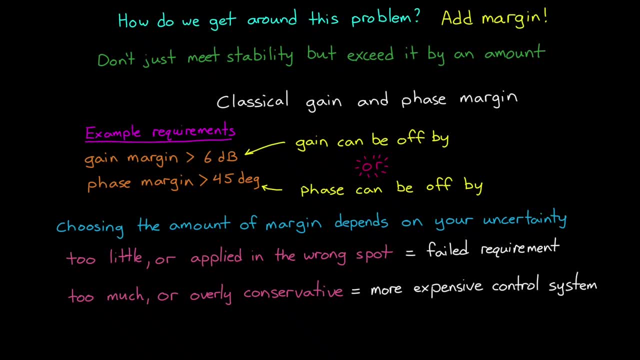 ourselves to build a system that has to meet more stringent requirements, And typically this results in a more expensive control system, either with direct hardware costs for sensors and actuators that have less noise or better performance, or it costs more in engineering time to design and test. 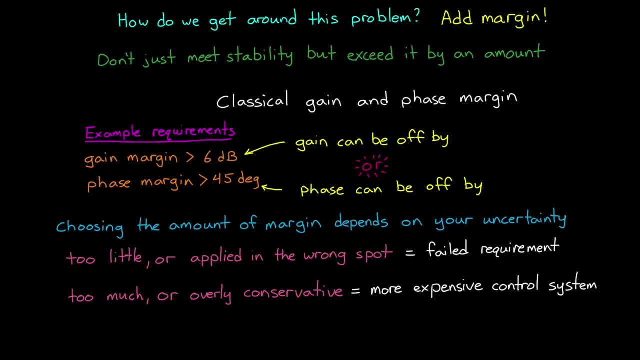 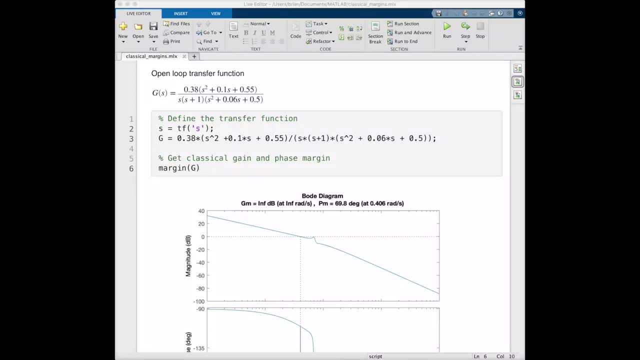 a higher performing system. So the trick is to choose the perfect gain and phase margin that fits the perfect amount of margin, and to apply it to the right places. And gain and phase margins are just one way to assess the robustness of your system And they're useful, for sure, but they don't necessarily. 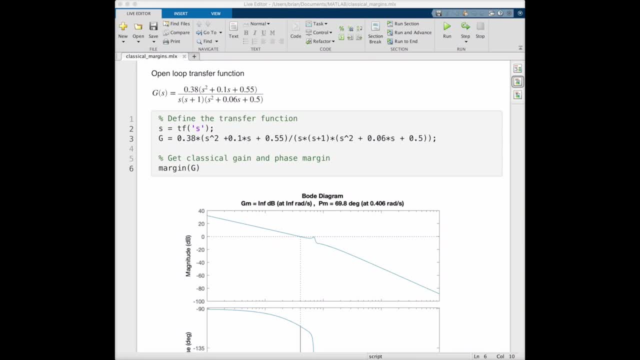 give a complete view of how robust your system is. For example, take this open loop transfer function G of S. I can solve for the classical gain and phase margins with the function margin in MATLAB And here you can see that this system has infinite gain margin, meaning no amount of additional gain. 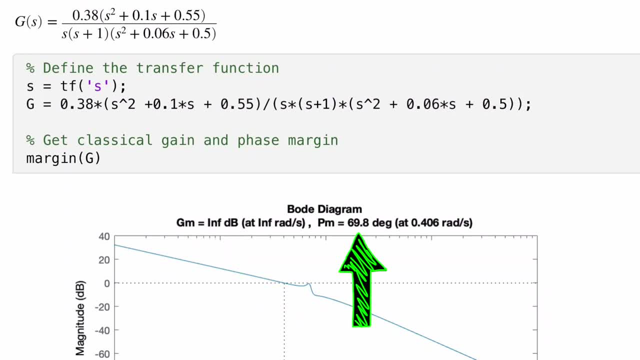 will make the closed-loop system more efficient than the normal gain and phase margin, And that's because the closed-loop system is unstable And it has almost 70 degrees of phase margin at 0.4 radians per second, which is equivalent to about 3 seconds of delay margin, So this feels like a pretty robust system. 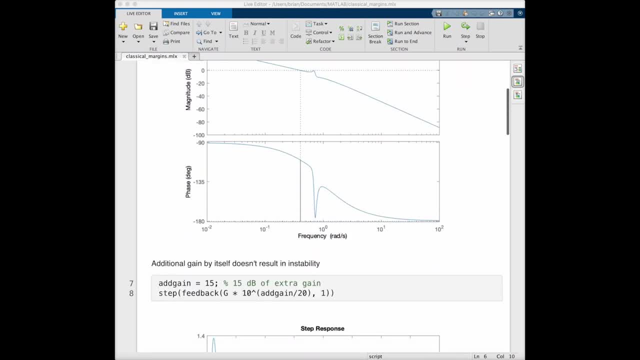 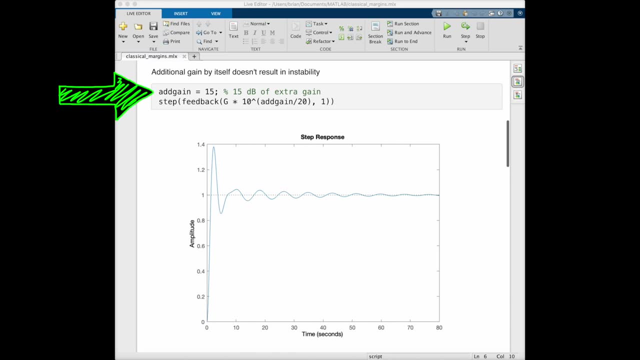 since it has such high margins, And to show this, let's assume that the gain in our model was way off and the real system has an open loop gain that is 15 decibels higher. We can get the closed loop system with the feedback command and plot the step response for the closed loop system And 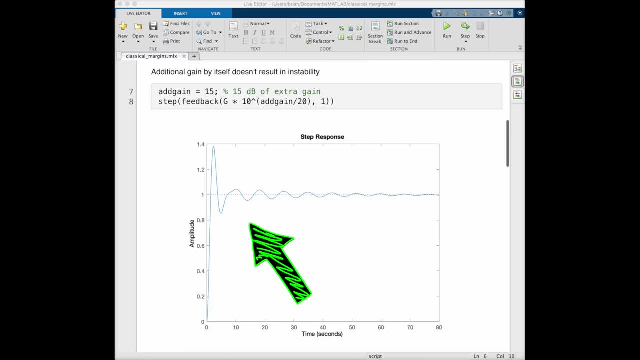 see that even with this large gain error, it's still a stable system. Now we can also add phase by itself by adding a delay to the open loop system. Here I've chosen a delay of 2 seconds and this eats up about two-thirds of the total phase margin And, as you can see, with the step, 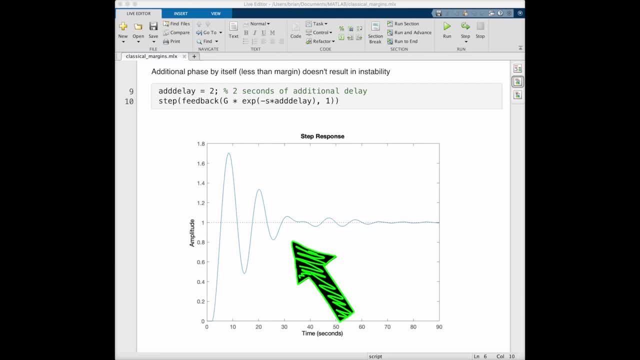 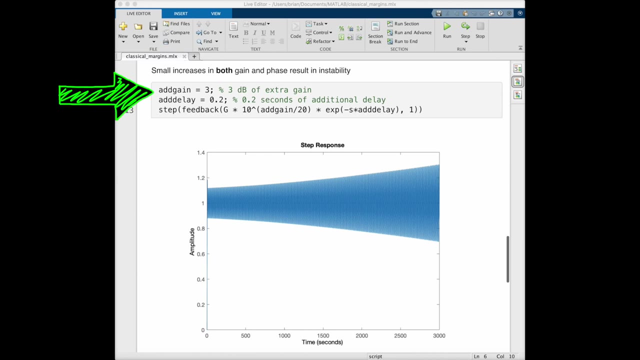 response. this closed-loop system is also stable. So a gain increase of 15 decibels by itself or an added delay of 2 seconds by itself are both stable variations. However, if we increase both the gain and the phase, then the story's different. Here I'm only adding 3 decibels of gain and a 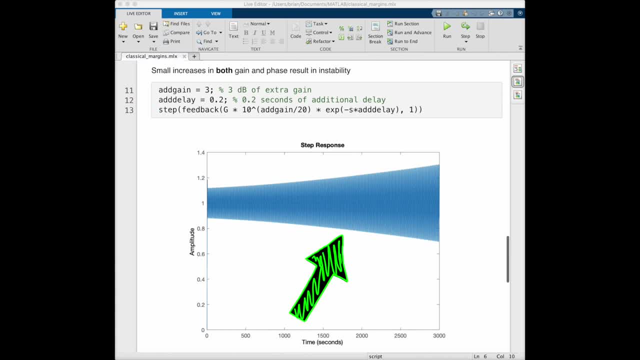 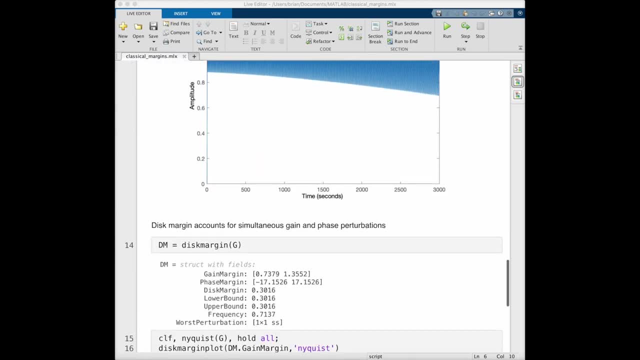 measly 0.2 seconds of delay, and this causes the closed-loop system to go unstable, So it's not as robust as we were expecting it to be. Therefore, the combination of gain and phase uncertainty also needs to be considered, and not just each individually. This is why we may look at disk. 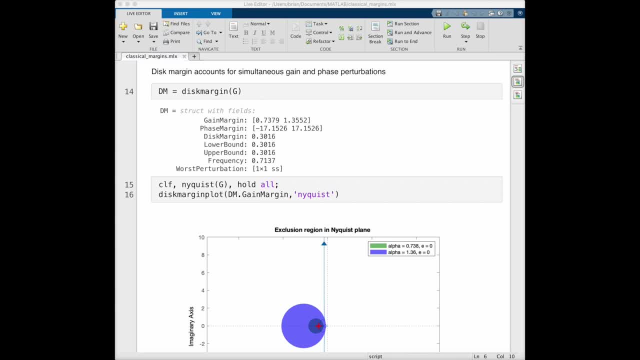 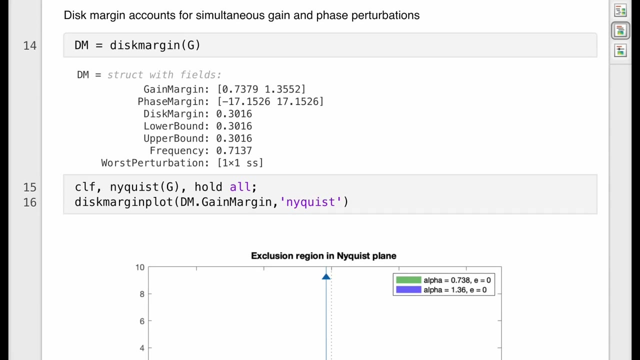 margin rather than classical margins, because it accounts for simultaneous gain and phase perturbations. Disk margins also have another benefit of being able to be applied to multi-input, multi-output systems, which classical gain and phase margins don't really handle very well. There is a lot to unpack here with all of these numbers. 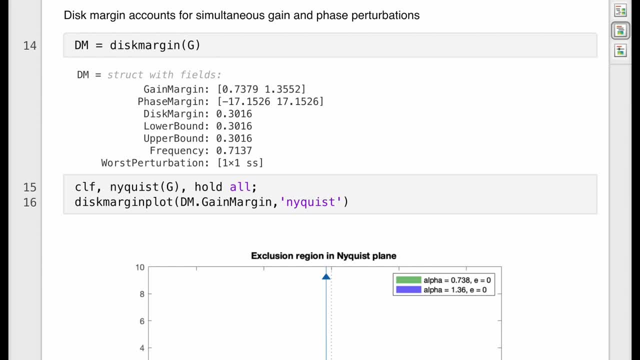 and we're going to talk more about disk margins later in the next video. But one thing to note quickly is that this is showing that the disk gain and phase margins are only about 1.3 and 17 degrees respectively, which aligns with our experimental results. So it's much less than 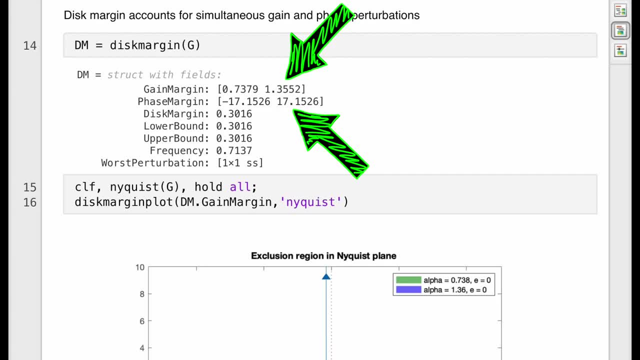 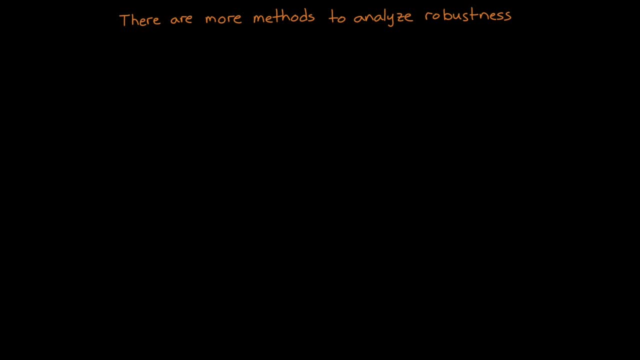 we're reported with the classical gain and phase margins. Now there are more methods to analyze robustness than just these two, But the general idea is the same for every method, which is figure out how much uncertainty and variation your system can handle before it no longer meets the intent. So, with that in mind, we need a way to represent 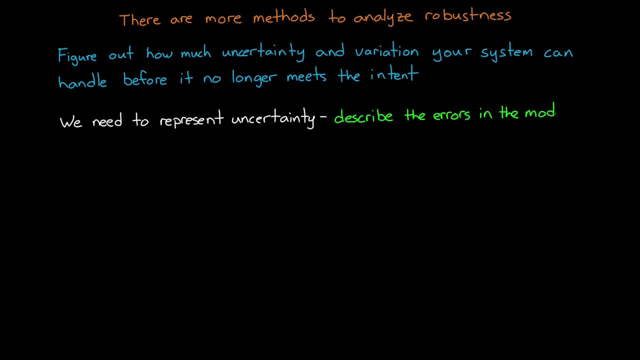 uncertainty. What I mean by that is how to describe the errors in the model or the differences between it and the real system. And this might seem a little odd at first, because if you knew where differed from the real system, why capture uncertainty? Why not just update the model? 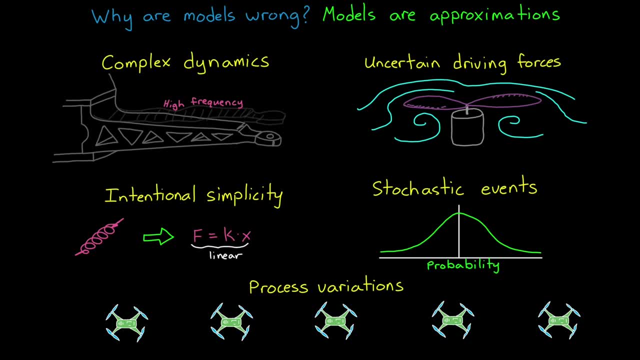 And the reasons were all of the reasons that I covered earlier. Often we can bound uncertainty without fully knowing the dynamics that are causing it. For example, we may not be able to predict sensor noise or vibration through some structure, but we can figure out that the noise 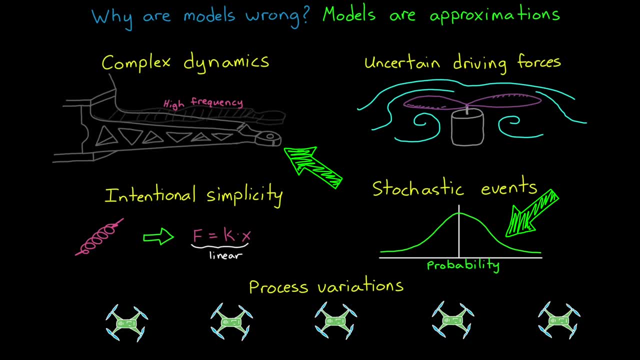 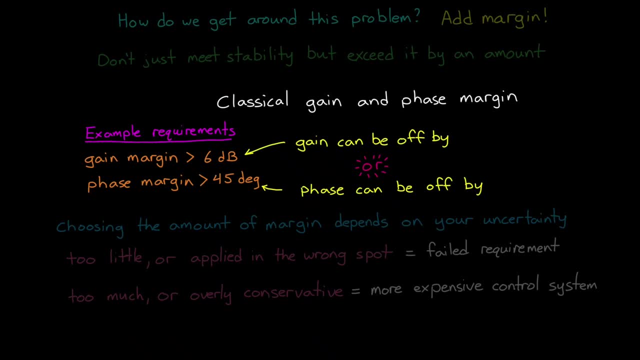 or vibration won't exceed some threshold or has some statistical probability distribution For classical gain and phase margins, we're representing our uncertainty as purely gain error or purely phase error, And when we say that we require 6 dB and 45 degrees margin, 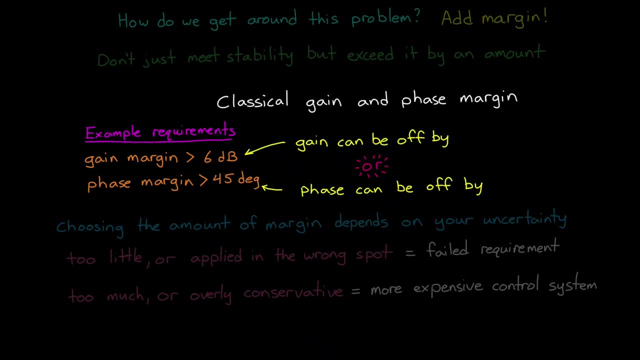 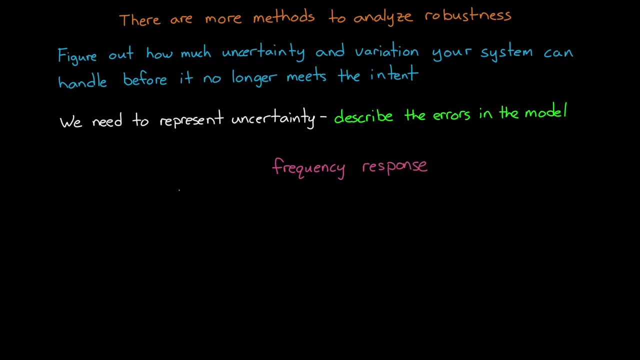 that means we've assessed our system and our model and believe the errors to be bounded by those values. But we can represent uncertainty in other ways. For example, the amount of uncertainty could be based on frequency. We might say that we have a lot more confidence in our model at low frequencies. 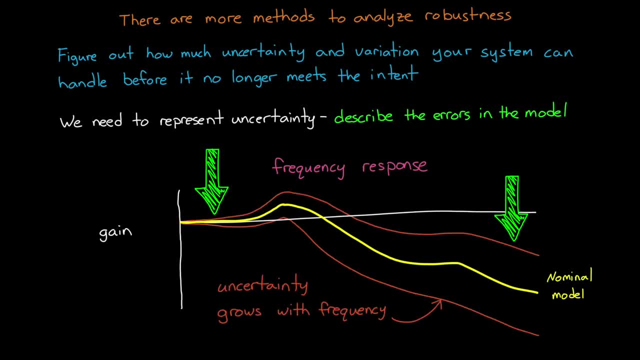 than we do at higher frequencies. We might say that we have a lot more confidence in our model at low frequencies, So we may require less margin in the design for low frequency behaviors while requiring more margin for high frequency behaviors. Okay, so far we've only introduced the analysis portion of robust control theory. 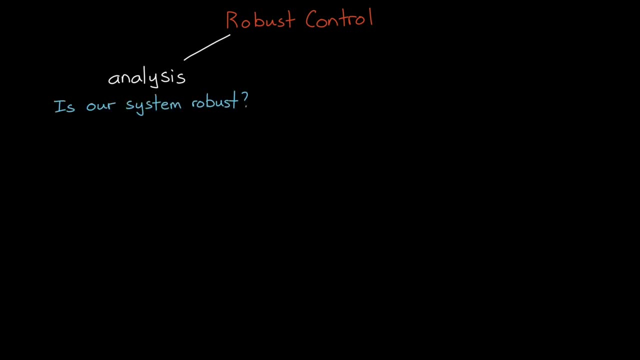 That's figuring out the system that we have. But the other half of robust control is synthesis, which is creating a system specifically with robustness in mind, or designing a controller that produces the needed amount of margin in the system. Now, the thing to note here is that robust control is not a specific type of controller, like PID or 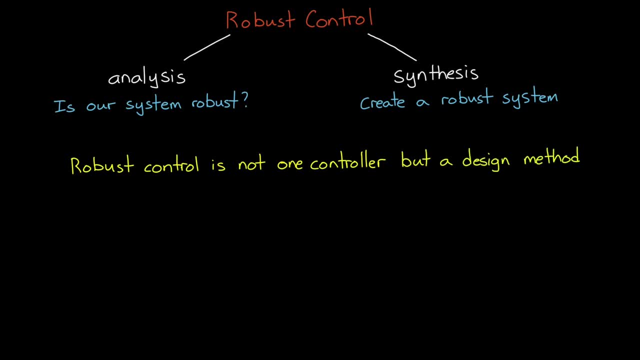 full-state feedback. Instead, it's a design method. It's a set of tools that allow us to choose PID gains or choose full-state feedback gains, or to tune some other controller so that it is robust. In this way, we can design, for example, a single PID controller using robust 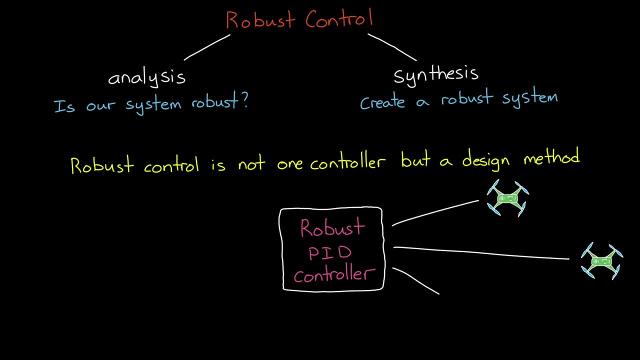 methods that will hover all of our toy drones And as long as the drone parameters or dynamics vary within the bounds of our understanding, we can design a controller that will allow us to choose PID gains or choose full-state feedback gains, or to tune some other controller so that 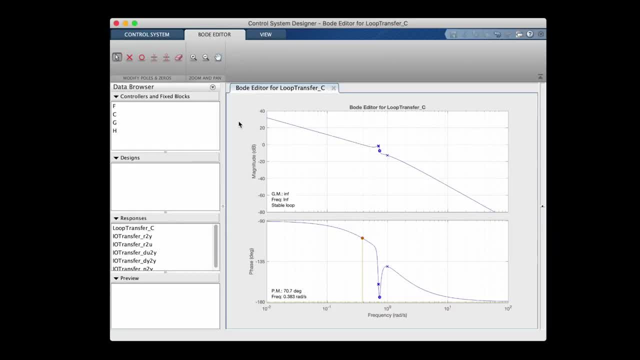 it is robust. In the classical sense loop shaping is a robust control method. We can set a specified gain or phase margin and then shape the loop by adding gains and poles and zeros until the design meets those requirements. But classical loop shaping becomes difficult for multi-input.